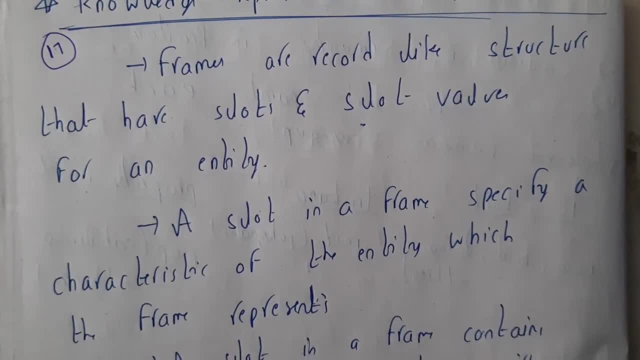 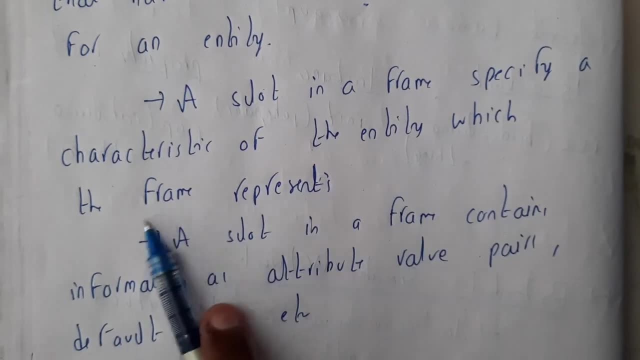 and inside that we will be writing the slot values. So once we are going through the example, you will be having a clear idea, do not worry. So a slot in a frame specifies a character of entities which the frame represent. A slot in a frame contains information as: 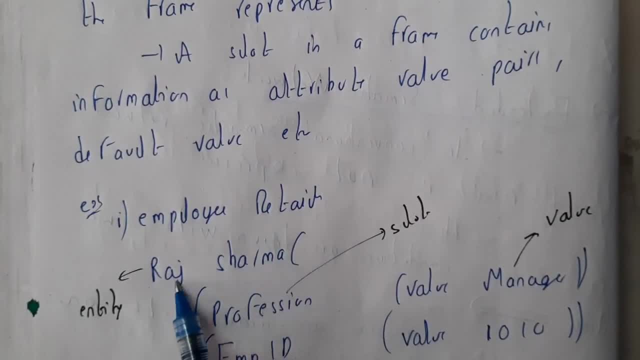 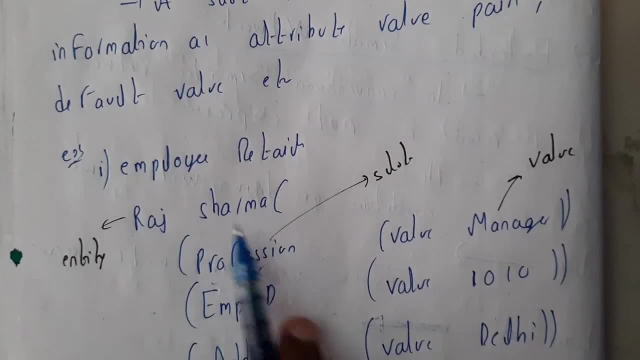 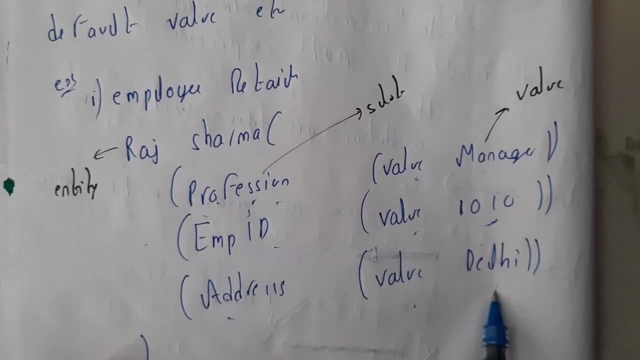 attribute value, pairs, default values. So employee details. the name is Raj Sharma, the guy name, So his E is nothing but the entity and the professor raj sharma, professor value, manager, employee id value, some value address value, delhi, like this. so this is nothing but a slot and this is the slot value, guys that this 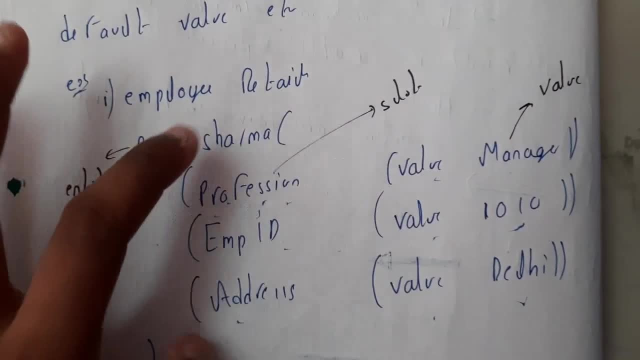 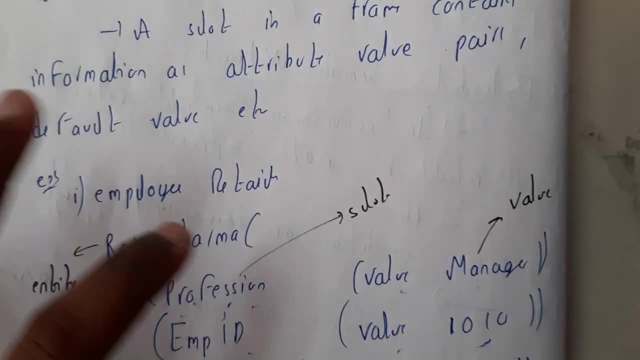 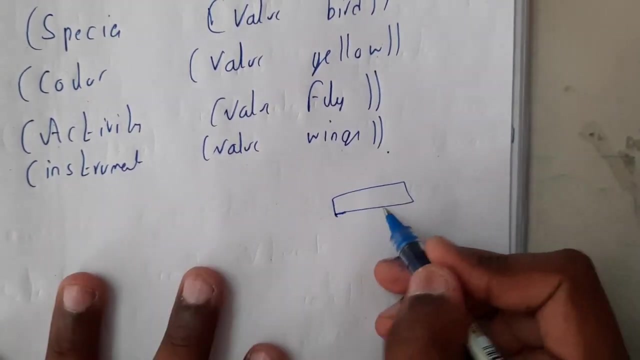 particular slots value is written here. that's it. so in this way we will be representing guys. so basically we can even represent this in terms of graphical also. so about raj sharma? or okay, let us assume you are having 100 employees. okay, so this will be your employee or your college name, or 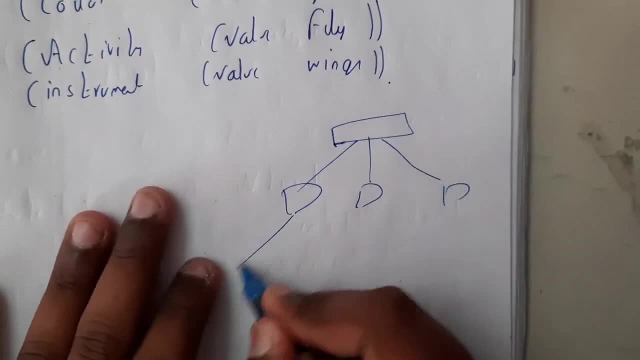 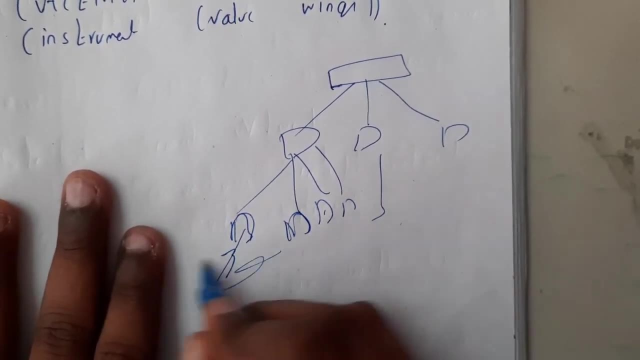 anything name. so in that, different, different departments, so each department is having the particular guys and the guys details like that. so the guys here till here, you will be having the graph, so you can even represent in the graph format: guys, guys, if possible. i'll be just searching for. 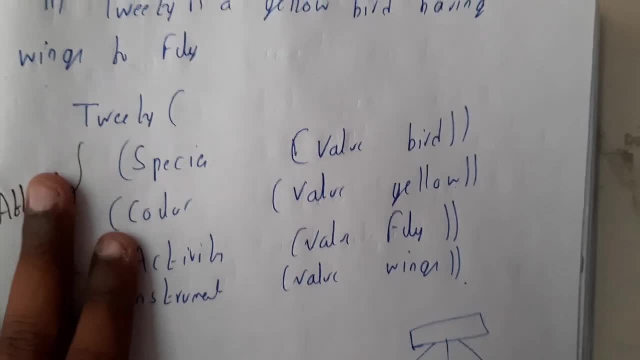 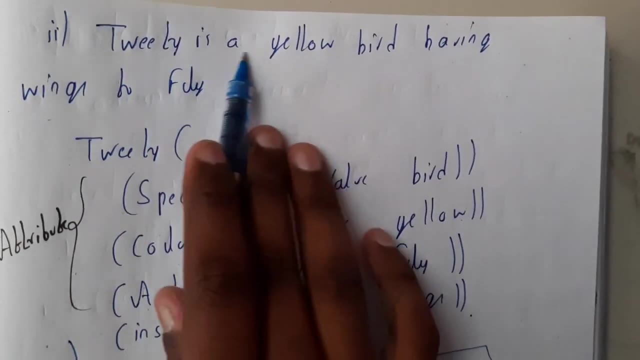 some frames- graphical plus normal representation, so that you'll be having a clear idea. so, similarly, if they gave a statement and they asked you to write it in terms of a frame, so you can write it in this way: twitty is a yellow bird having the wings to. 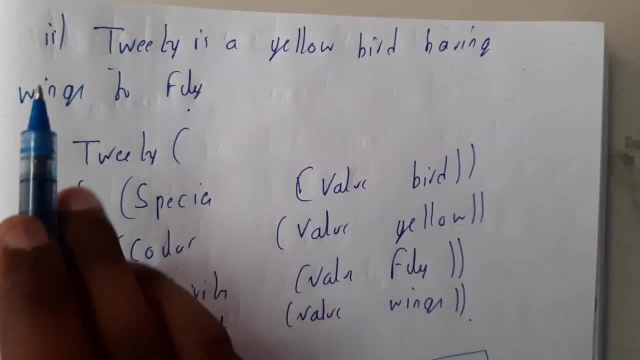 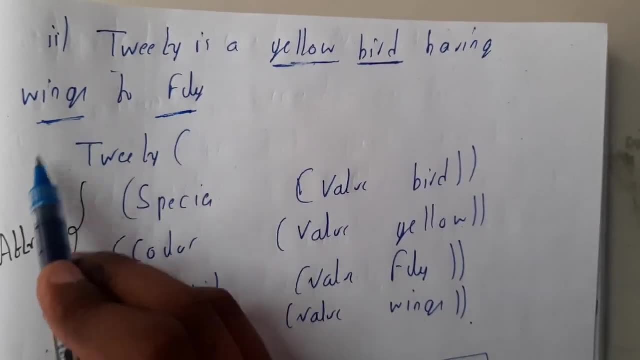 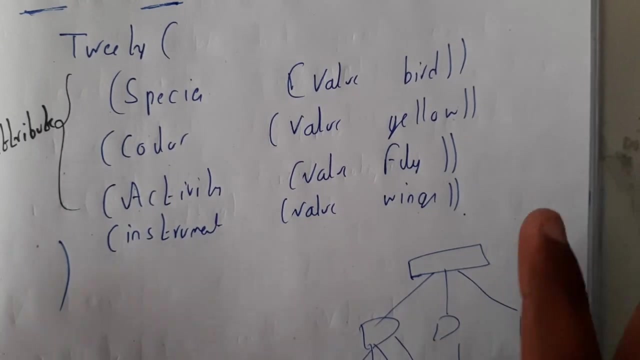 fly. so what are the different things, guys? twitty is the bird name, that's fine. so it is: color is given, its species is given, it says that it is having a wings and it says that it can fly. so twitty species value, bird color value. yellow activity value, flies instrument: how it is flying. 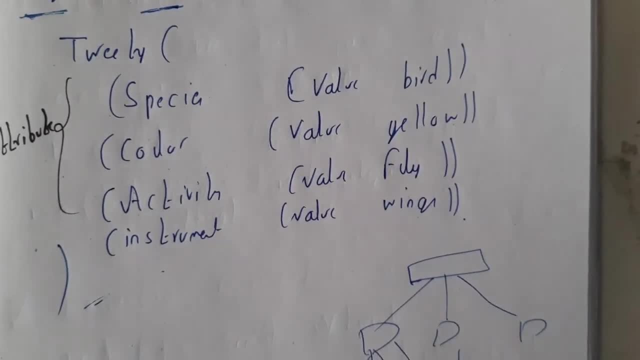 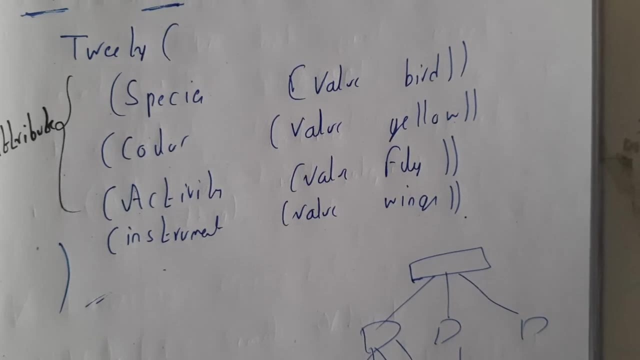 guys with the help of wings, so instrument wings. so in this way you can represent guys. so i hope everyone got a clear idea on this. so in the next lecture- by this we are completing the second unit, guys. so in the next lecture we'll be going through some important topics of this chapter. thank you, thanks for watching.